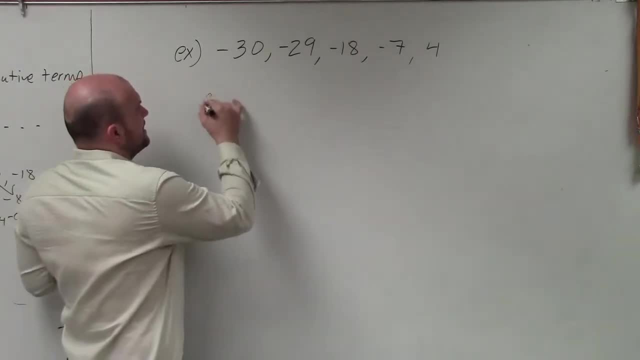 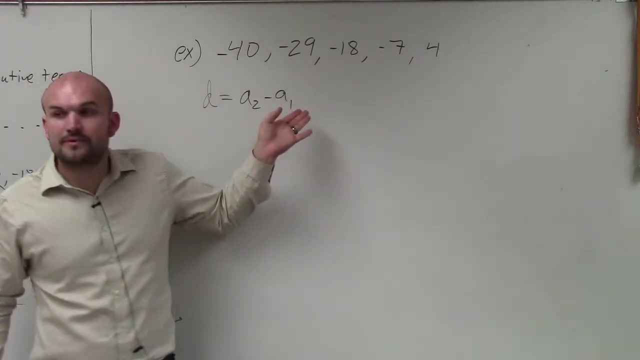 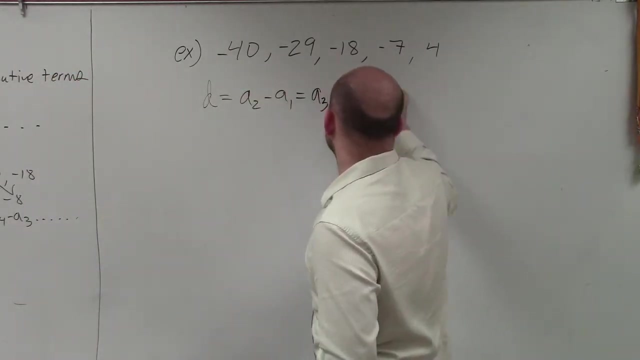 can be pretty difficult. So, as I mentioned, if you guys remember the rules that I said, the common difference is basically a2 minus a1.. No, that's supposed to be 40. So, if you remember, the difference is a2 minus a1 has to equal a3 minus a2, which has to equal a4. 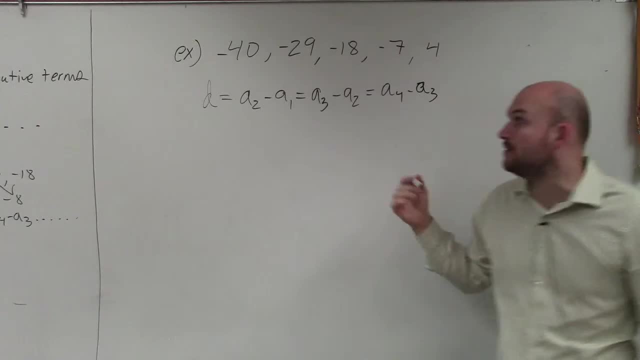 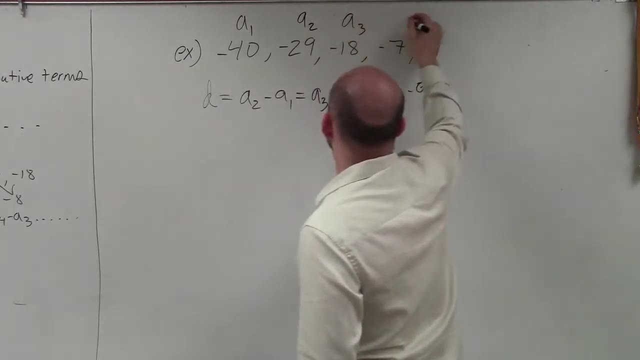 minus a3, and keeps on going and going. So we know that a negative 40 is a1.. Negative 29 is a2.. Negative 18 is a3. That's a4 and a5. So we got to also say that a5. 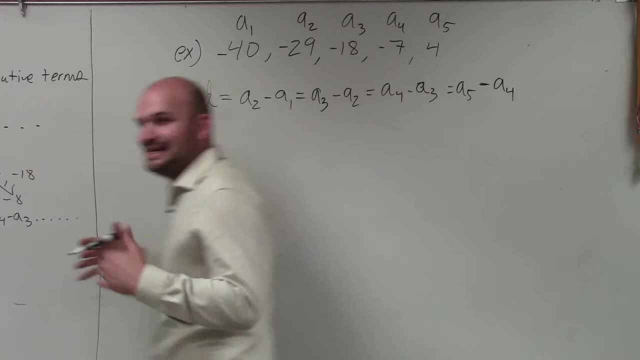 minus a4. And all of these has to equal the same value, which is d. So if we're going to plug these in here, I'm just going to do one and I'm going to verify to make sure that's the same for all of them. So if I did negative 40 minus a negative 29,, make sure you notice. 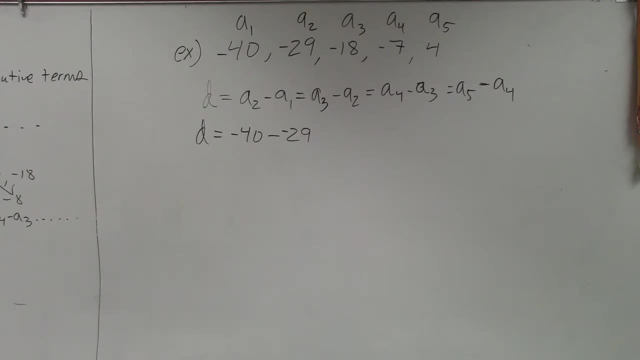 that that's a negative 29. So I'm taking negative 40 minus a negative 29. So I'm taking negative 40 minus a negative 29. So I'm taking negative 40 minus a negative 29. So I'm taking. 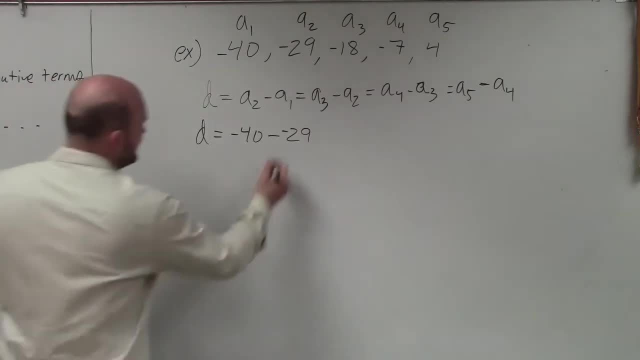 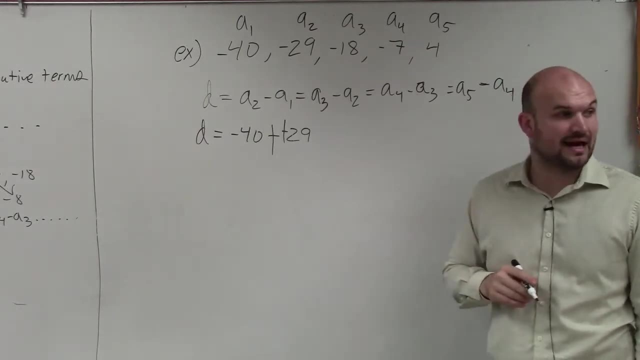 minusing a negative 29.. Well, since I'm minusing a negative, that becomes a positive, So it's really negative 40 plus 29,, which just gives me a negative 11.. So my difference is negative 11.. A lot of students will make the mistake and put a positive 11. And let's just make. 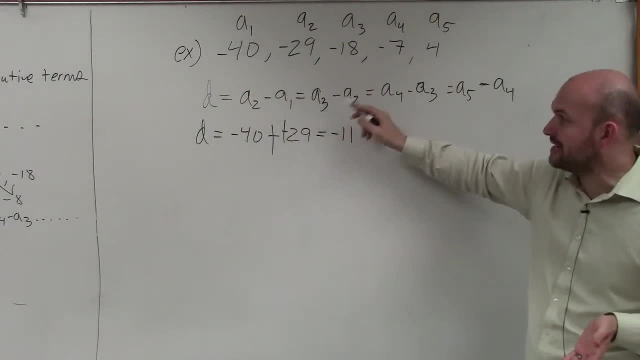 sure that is correct. I could do that, for I could do the same. I could subtract a3 minus a2.. I could do all of these, But let's just verify To go from 29 to 11, I'm going to. 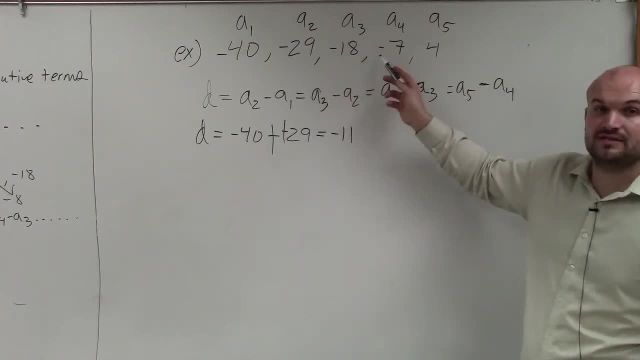 take a negative 11.. Does that have a difference of negative 11? Yes. Does that have a difference of negative 11? Yes, Oh shoot, You're right, You're right, You're right. Thank you very much, Actually, I'm. 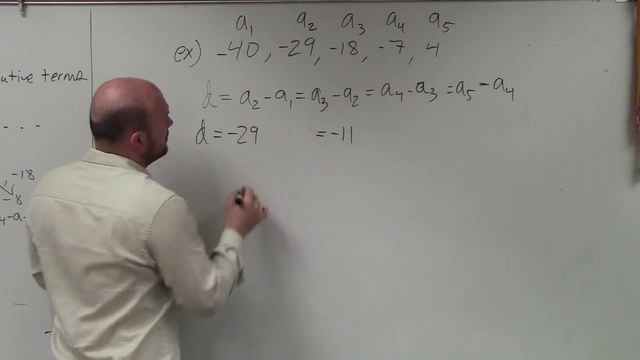 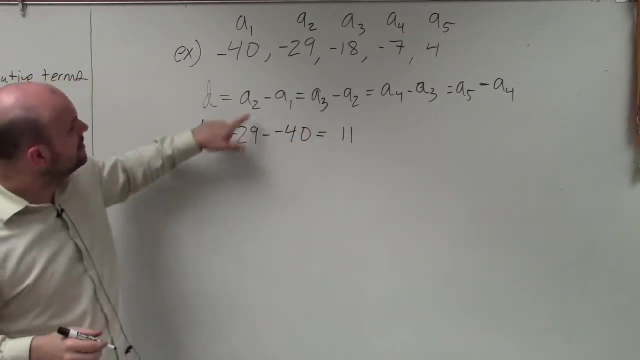 sorry, You're right, because that would be a positive. So it would be negative 29 minus a negative 40. So we're going to subtract, excuse me, So you're going to subtract negative 29 minus a negative 14, right. 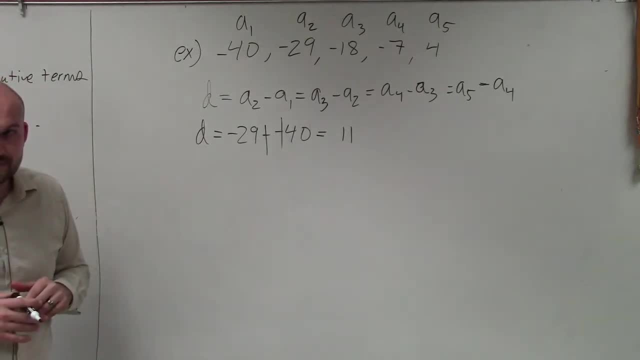 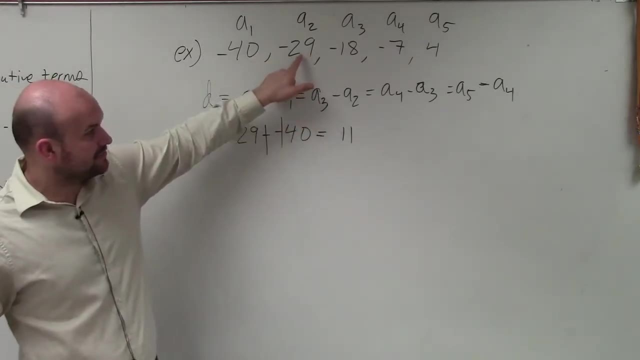 40, same thing that does become a positive. so therefore, that is going to be a positive 11, which actually would make more sense because if we're adding positive 11 to negative 29, we'll get negative 18. if I add 11 to negative 18, I